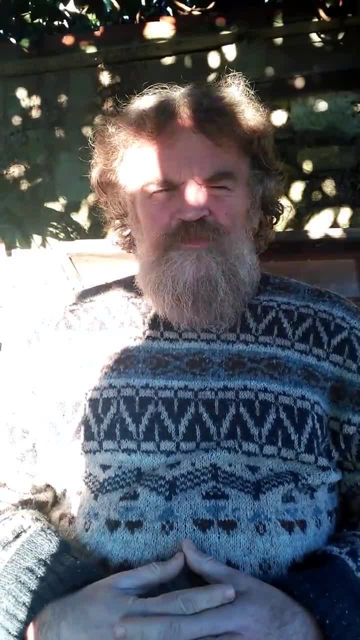 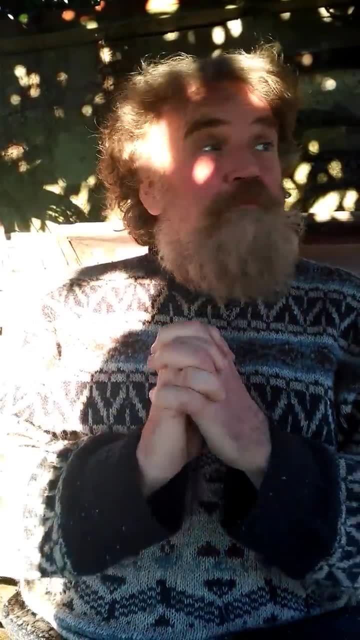 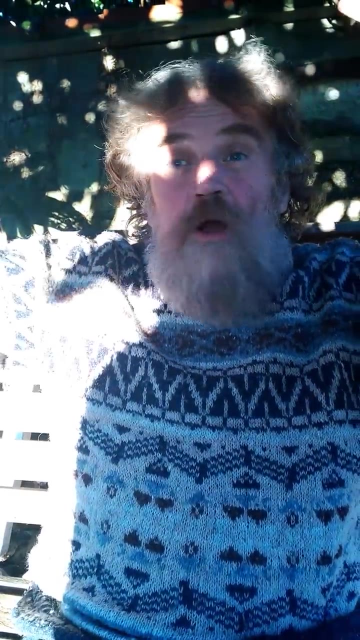 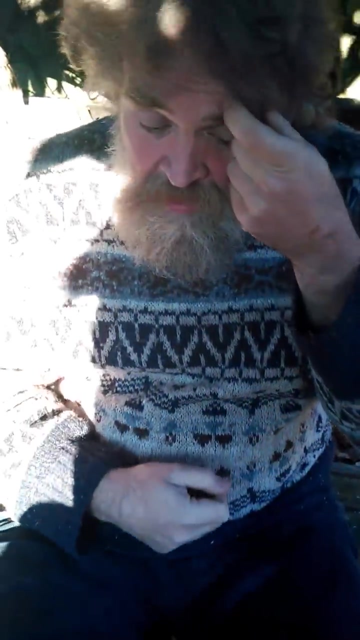 Hi there, students, To grovel- Okay to grovel is to beg, To beg on hands and knees. Please, please, please, please. Okay To grovel to bring yourself down in status and level, asking for something He will give: the boss will give you a pay rise, but you're going to have. 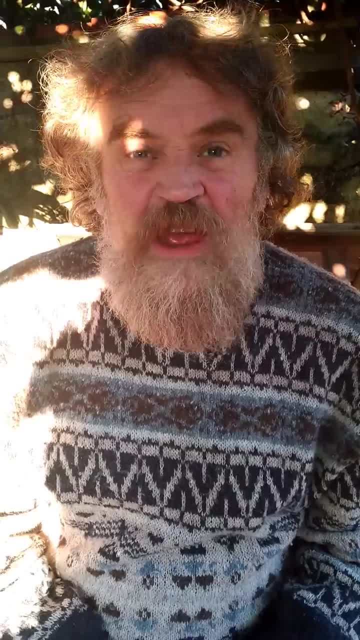 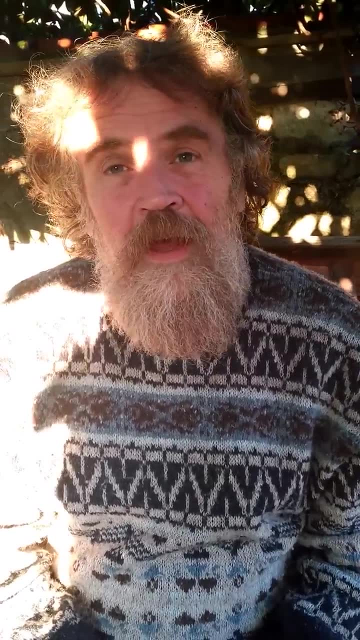 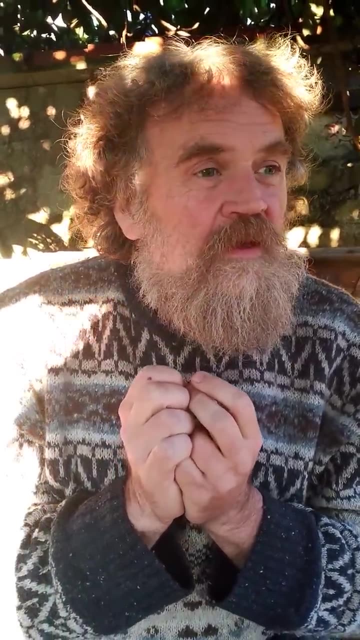 to grovel: Okay, You're probably going to need to ingratiate yourself with him. with him, Kiss his arse a bit. Suck up to him. Yeah, Be sycophantic, Okay, But grovel is really quite informal. Yeah, Okay To grovel is what you're going to have to do when you. 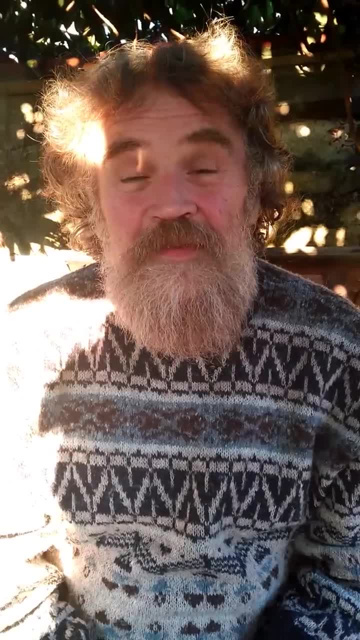 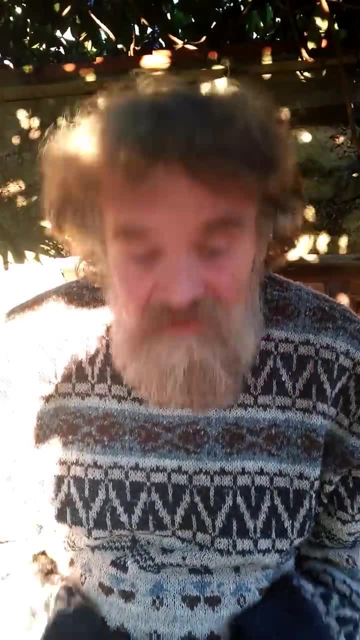 ask your worst enemy For a favour. Yeah, Yeah, He's not going to just say, sure, why not? No problem, You're going to have to bring yourself down in status to be humble, to humble yourself, Okay So. 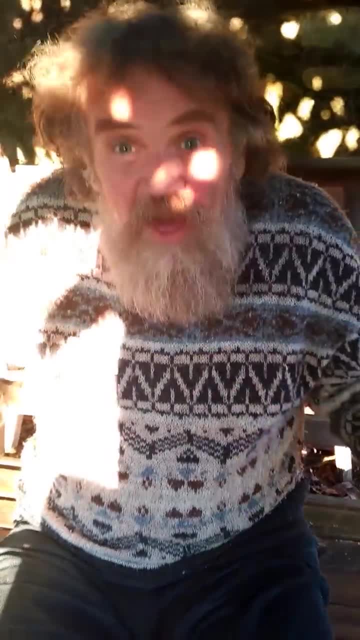 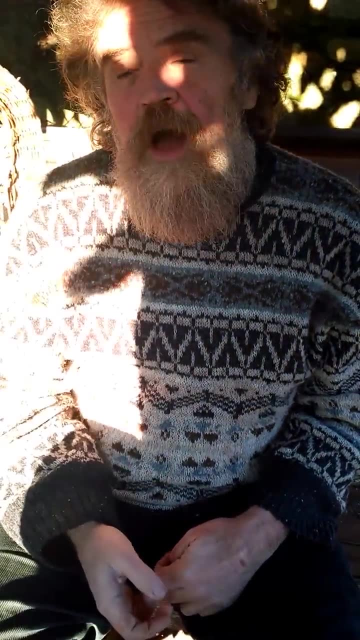 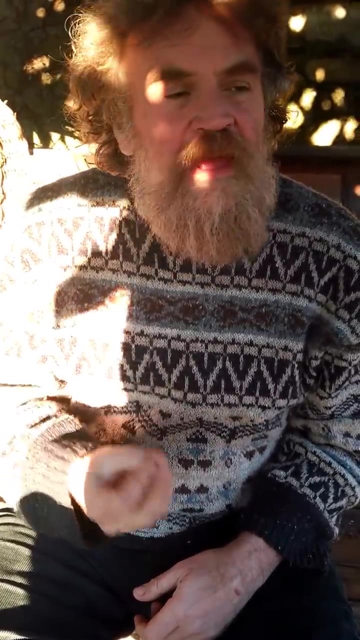 when you grovel- yeah, you've got this idea of almost lying on the floor. Please, please, please To grovel to somebody. Okay, We use this as well in the idea of to be sycophantic. Um, he's always groveling to the boss. Yeah, He's kowtowing to him, if you like. Okay, So 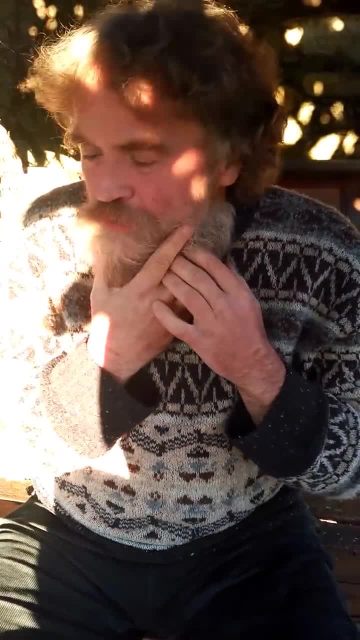 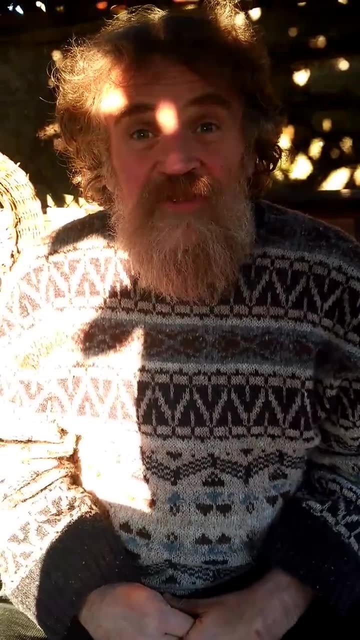 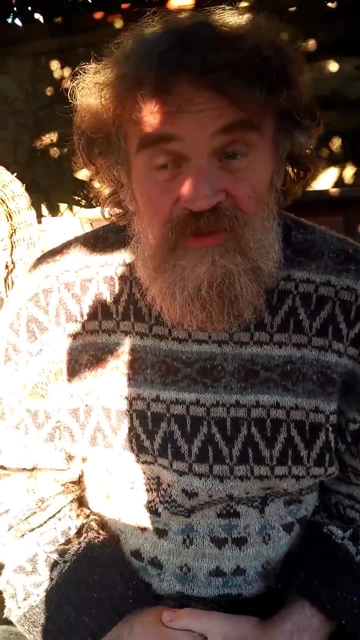 to grovel? Yeah, Please, But by rebasing yourself to the lowest level. Yeah Okay, He groveled in the mud so that his boss could walk over him. Yeah Okay, All of these people are always groveling to their bank manager. Okay, Stop groveling. Yeah, There's no need to grovel. 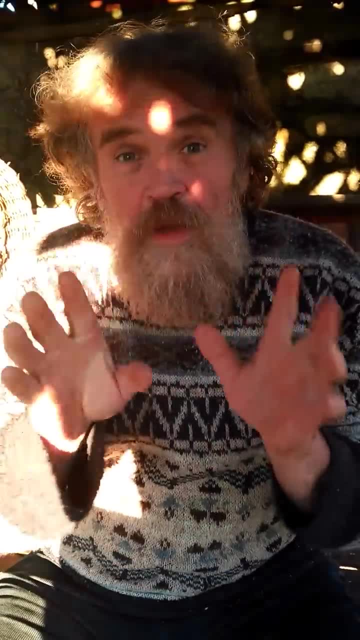 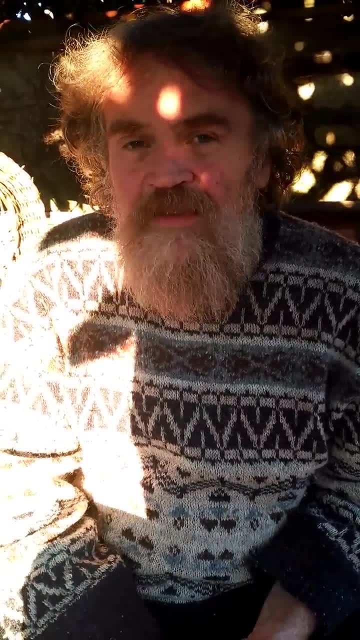 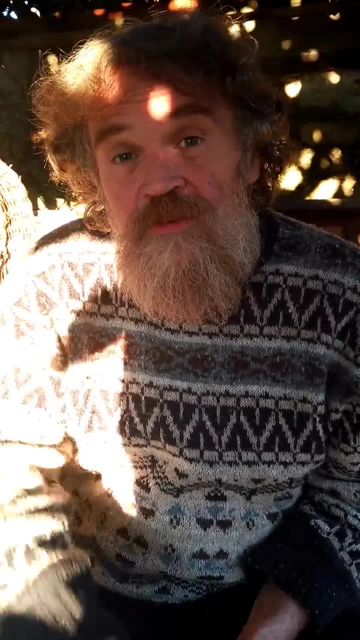 if you enjoyed the video, give it a rating. You can make a nice comment, but don't grovel, It's not necessary. Um subscribe to the channel and I'll see you soon. Bye for now.